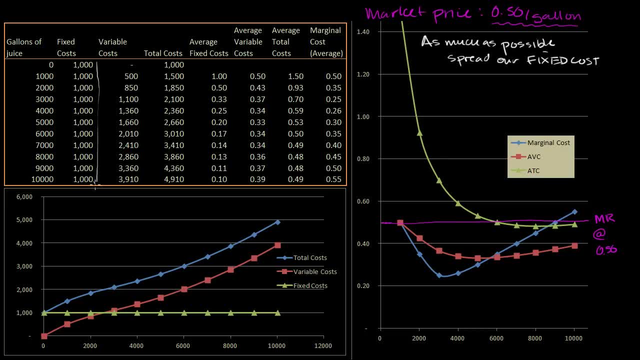 We are spending $1,000 no matter what. So why don't we try to get as much revenue as possible to try to make up for those fixed costs? Or if we think about it in terms of average fixed costs, the more quantity that we produce. 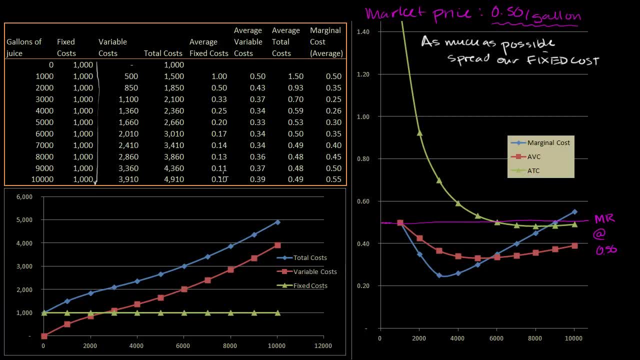 the component of the cost for that from the fixed costs go down and down and down. So we want to have as much as possible to spread our fixed costs. Now, the one thing that we do need to think about is especially once we kind of get beyond this little dip. 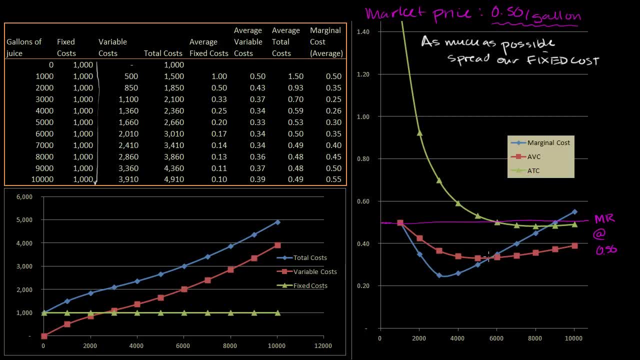 in the marginal cost curve and as we're producing more and more units, the marginal cost is going up higher and higher and higher. we don't want to produce so much that the cost of producing that incremental unit, the marginal cost of that incremental unit. 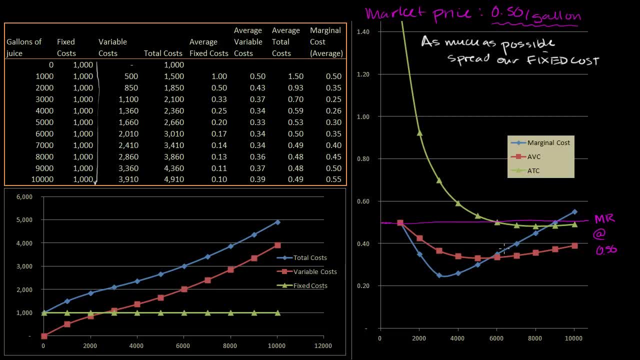 is more than the marginal cost of that actual or the marginal cost of the fixed cost, The marginal cost of that incremental unit is not higher than the marginal revenue that we're getting on that incremental unit. So until marginal revenue is equal to marginal cost, 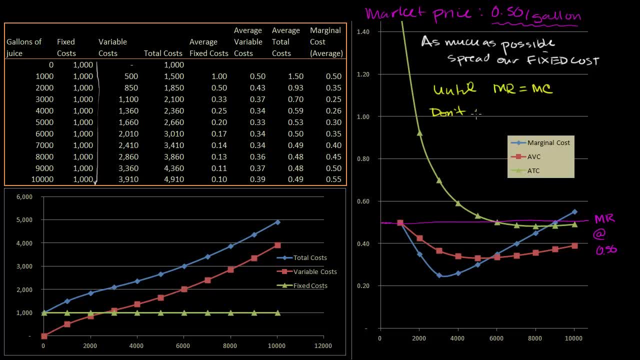 or another way of thinking about it. you don't want marginal cost, and this is after we go through this little dip here. We're trying to do as much as possible. Marginal cost is going higher and higher and higher. We don't want to produce this much. 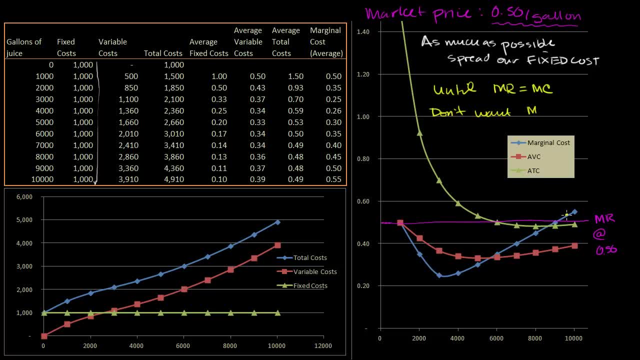 right over here, because here that cost for that extra gallon is higher than what we're going to get for that extra gallon. Looks like that cost for that extra gallon might be $0.53, while we're only going to get $0.50 for that extra gallon. 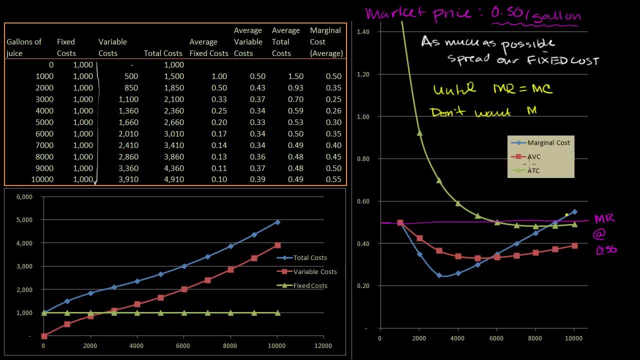 So every extra gallon we produce over here we're going to be losing money. So you don't want marginal cost to be greater than marginal revenue. So when you look at the curves like this, it makes sense to just say: well, when does marginal revenue equal? 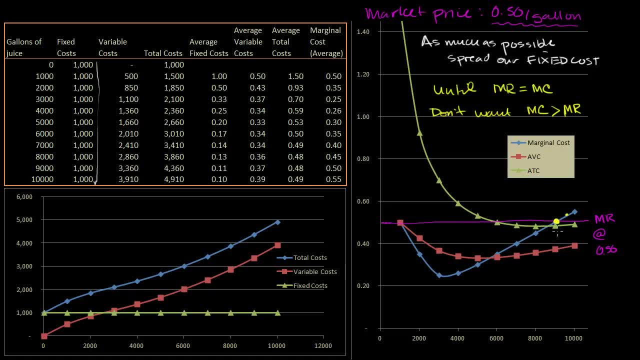 to marginal cost, And that's this point right over here, and that is the rational amount to produce. So that is 9,000 units. So we're going to be at this line right over here, We're going to produce 9,000 gallons of juice. 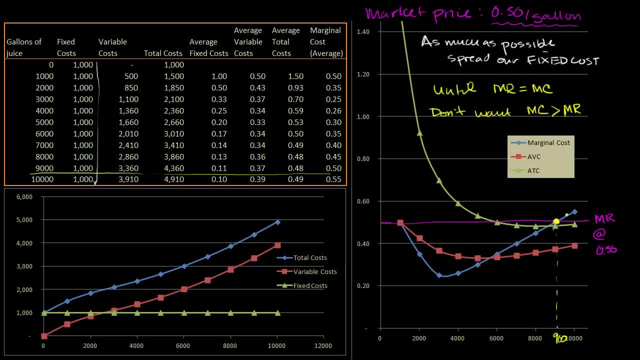 Our revenue that we're going to get is going to be the area is going to be the rectangle of the area. that's as high as the price we're getting per unit times the number of units. So this is going to be the total revenue we get. 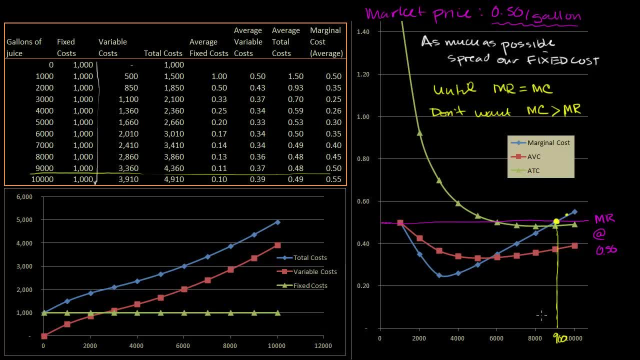 if we were to shade this in- and I'm not going to shade it in because it's going to make my whole diagram messy. And what is our total cost? Well, we have our average total cost right here. Our average total costs are $0.48.. 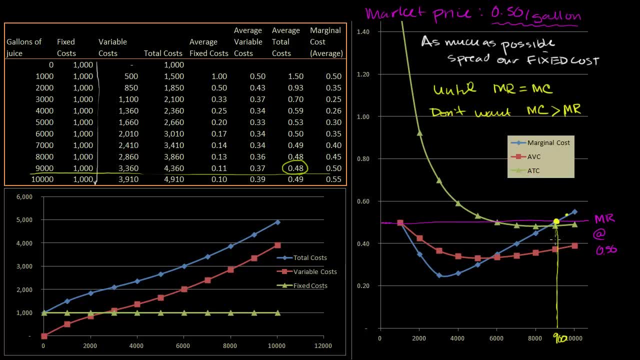 That's this little green triangle right over here. So it's $0.48 per unit times the total number of units. Our costs are the area under the area in this rectangle. So if I were to shade this in this little slightly smaller. 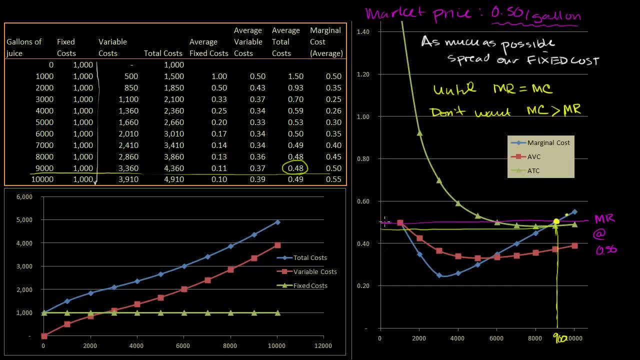 rectangle, And so our profits are the difference between the two. Our total revenue is the area. It's the area under the rectangle that has the marginal revenue line as its upper bound, And our cost is a rectangle that has our average total cost. 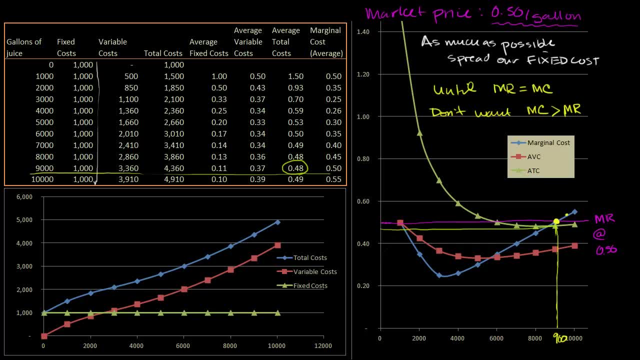 this line right over here as its upper bound. So our profits in this circumstance are going to be the area right over here. The height is the difference between our marginal cost, which is the same as our marginal revenue, and our total cost. So the height is going to be these $0.02 right over here. 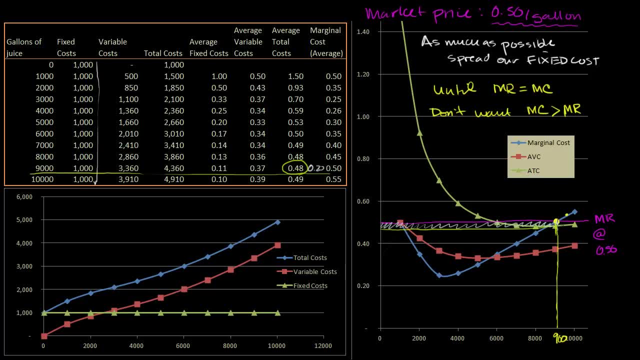 We're taking the difference between the two, $0.50 and $0.48.. So it's going to be $0.02.. And then the quantity produced is going to be 9,000 units. So 9,000, we're making $0.02 per unit. 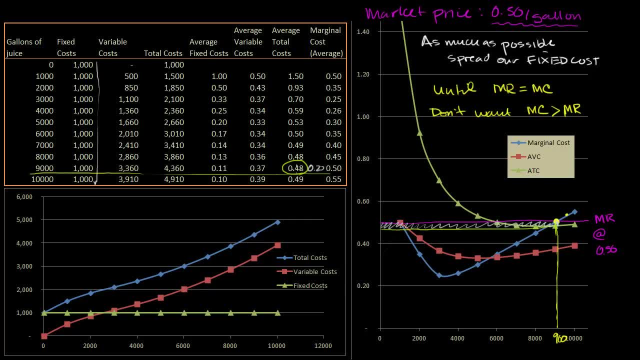 Remember, our average total cost is $0.48 per unit. We're selling them at $0.50 per unit, So we're making $0.02 per unit. I wrote $0.20.. We're making $0.02 per unit. 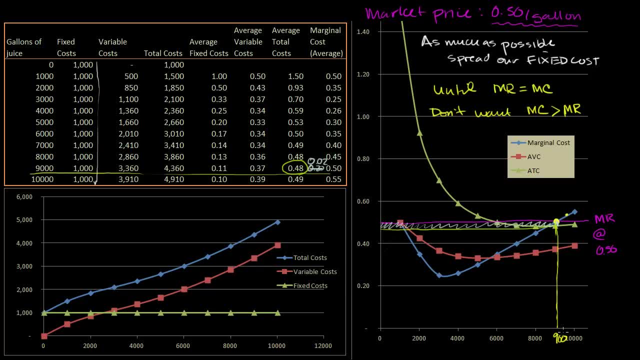 $0.02 times 9,000 units gives us what is that? That's $0.18.. Or $180 of profit. Now what I want you to think about- and we'll answer this in the next video- is: does it make sense to sell units at all?